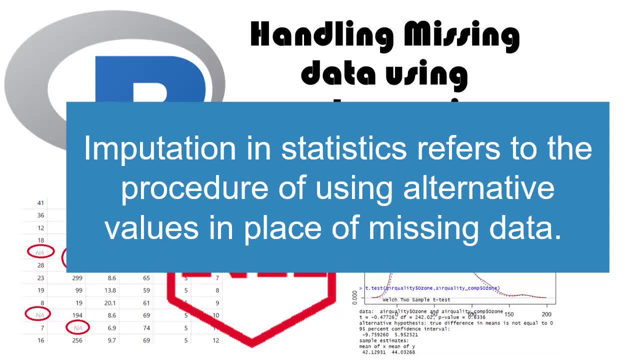 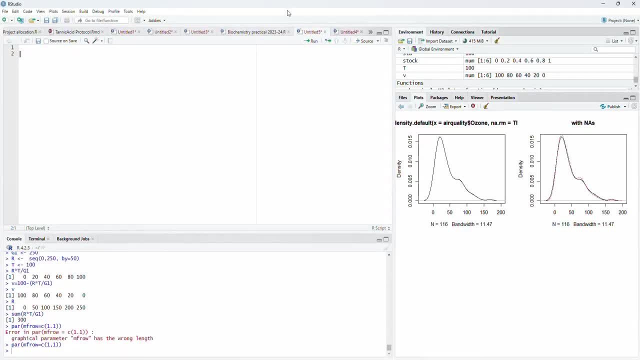 To impute our data. Data imputation is replacing the missing values with the most probable values which are there. We will first see how to visualize the missing data and we are going to use air quality data to learn the data imputation. Air quality data set is the data set which contain many missing values and is a very popular data set to learn how to handle missing data And I have used the view function. 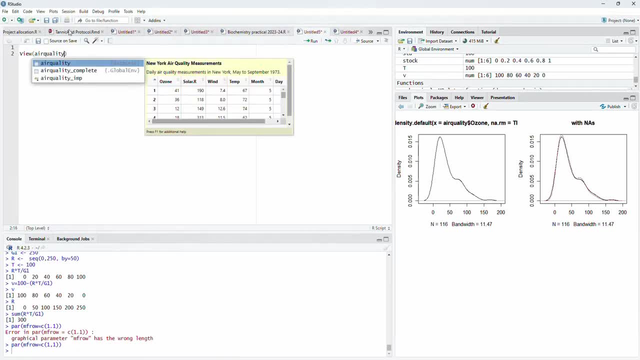 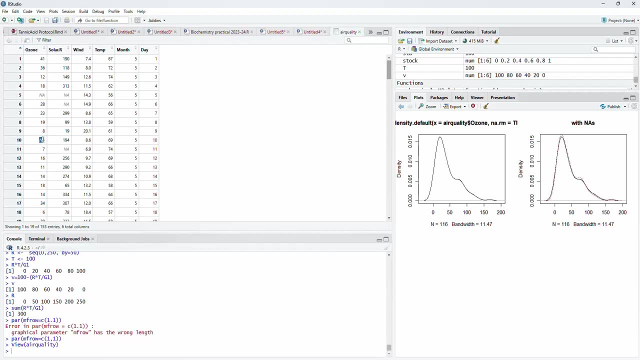 Air quality, And please remember that this V is uppercase. And when we see that, we will see a spreadsheet like visualization and these NA values are there. These NA values are there in ozone and solar R. These two columns and many NA values are there. Now we will see how to visualize those NA values and for that I am using the package. 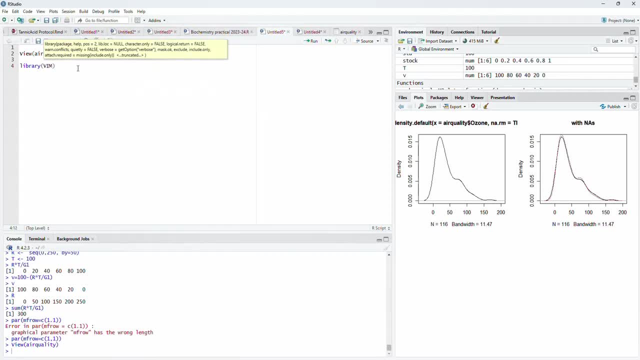 Library Vim, And if you are not installed package Vim, you can go to tools- install packages and type in package name Vim there And package will get installed. or alternatively, you can use installpackages- installpackages and type the package name in inverted quote Here the dialog box is open. I will type the package name. 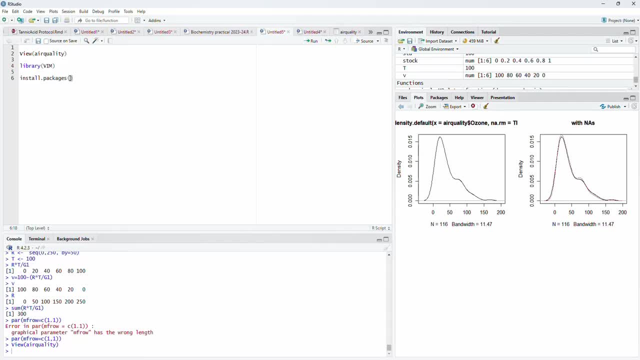 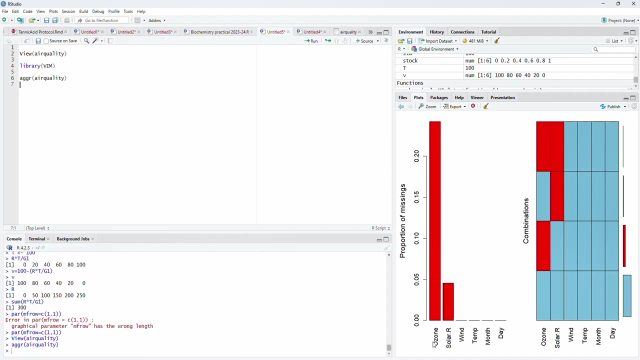 And click install, package will get installed. or you can put that name here and run this line: package will get installed. I have installed it. I will not run this line And the AGGR function of package. Vim visualize the data air quality and run that And you can see here that almost 24% of ozone is missing and around 0.5- around 5% of ozone is missing. 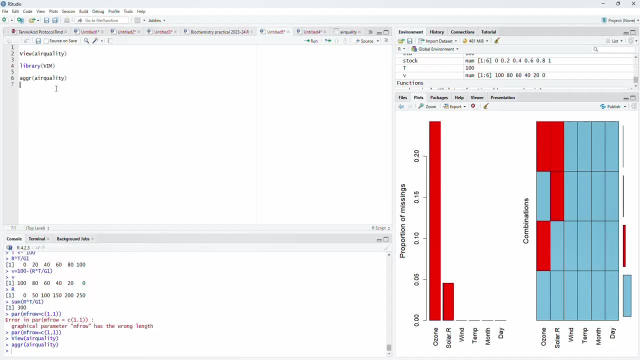 And if you omit these, we can omit that. We will see how many rows are getting omitted. End row NA dot omit. This function omits the missing data and you will get the rows with complete data only. We will run that 111 rows are retained and total rows of that. 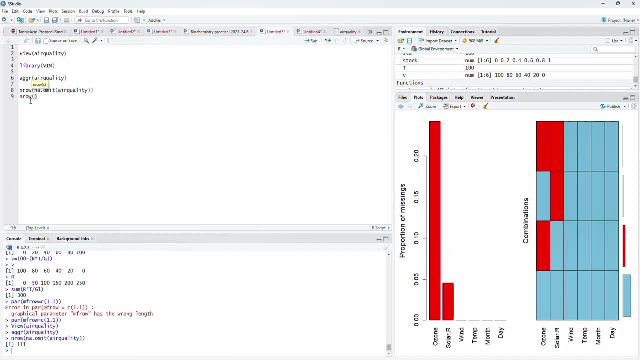 Air quality data are 153.. We will see that and 42 rows are omitted, And we cannot afford omission of these rows because we lose much of our data. Around 24% of the data will miss And for that purpose we need imputation. 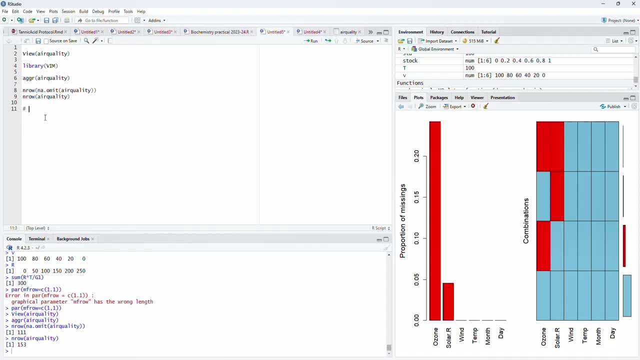 And for that we are going to first learn how to use Functions from package mice And I will call library mice for that, Library mice. If you have not installed mice you can install through tools Install packages, Type in package name there, Click install, Or you can have that install dot packages also, And I will run this line. Now library mice is there And I will give the name to the imputed data: that air quality. 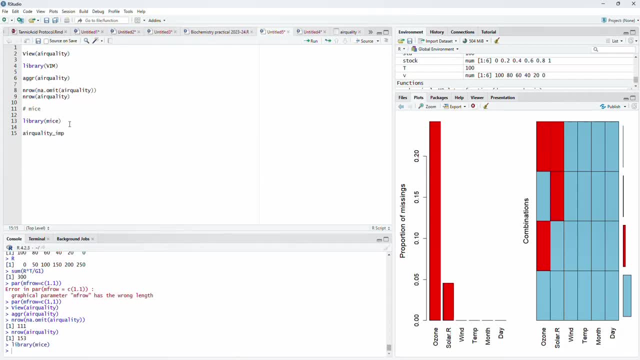 Underscore imp And use the function mice. When you type mice, you will get this tooltip text. This is the help for the mice function. The first argument is the data: M is 5 means 5 iteration you want or 5 different imputations you want to carry out. Then method is equal to none. Many different methods are there And by default that method is PMM, That is, predictive, mean, matching. 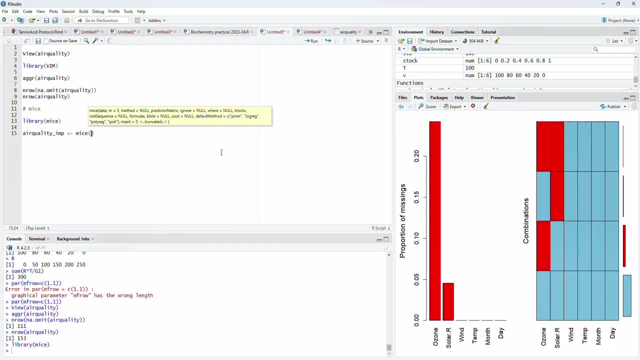 And other things are not much of importance to us Here. default method: PMM is there. Log rate, poly rate, Wherever required. it will select the method according to the characteristics of that data. I will type the dataset name here. I will not specify the imputation method: air quality. We will run that And you can see that iterations have taken place and we have the imputed data And we can see the structure of that imputed data. we have the expected sound and results and every result нам. 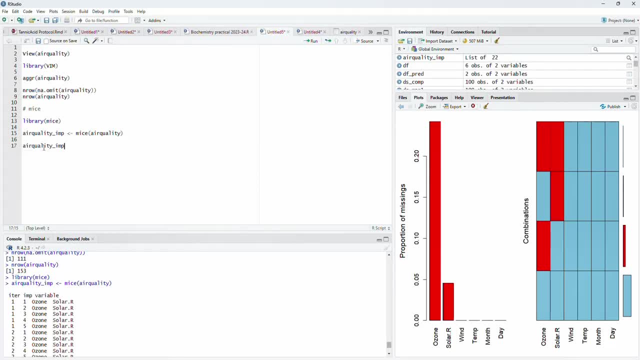 data also, and for that we will use the attributes function, attributes: air quality, in. we can see that their names are there, this data is there. imputed data sets are there, m, how many iterations are there and all those things. we are not going into details of those now. we will see how to get. 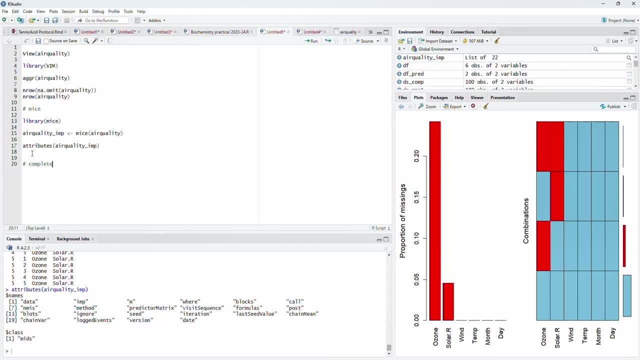 the complete data. we have to use that complete function for that air quality- complete. I will give the name and their complete function. we will use complete and in bracket we have to provide this imputed object, air quality, in give that and run that. now, complete data is there. now we see whether this is complete data or not. again using a GGR function. 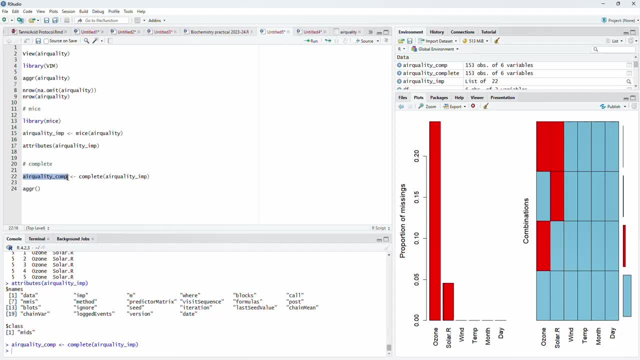 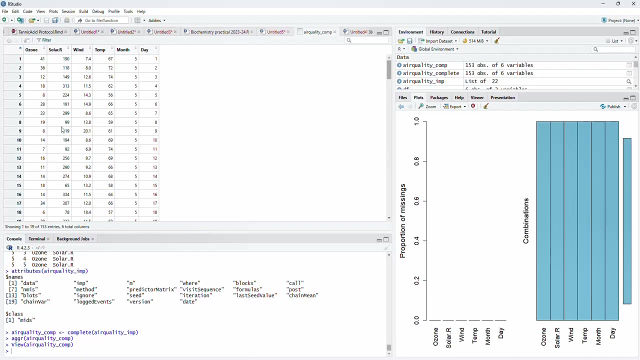 and to this a GGR function. this complete data will provide and you can see. the missing data is not there. it got imputed. we can view the imputed data also air quality in. will paste there and will run that and you can see that data imputation has taken place. no, any values are there and most probable 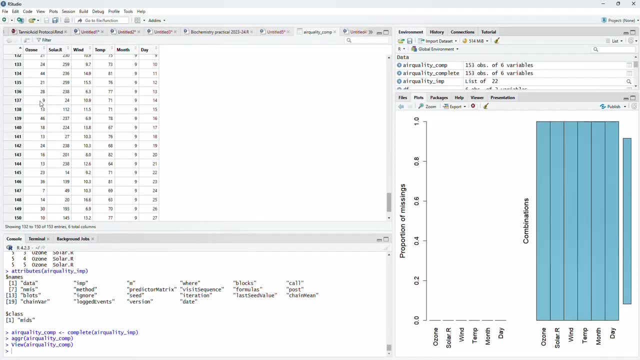 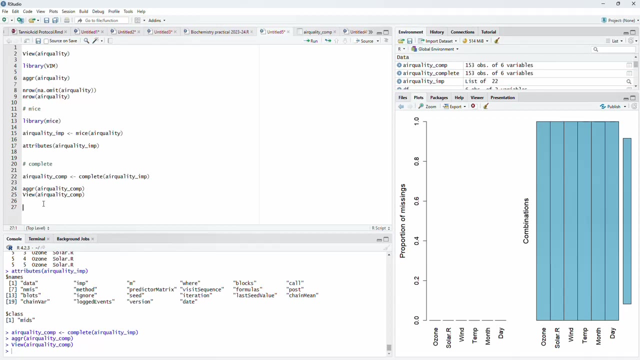 values which should be there if data was not missing. those got substituted for the missing values. now we will visualize the original data with missing values and imputed data to compare those, whether imputation has taken place properly or not. for that we are going to use just I will change the power so that we will. 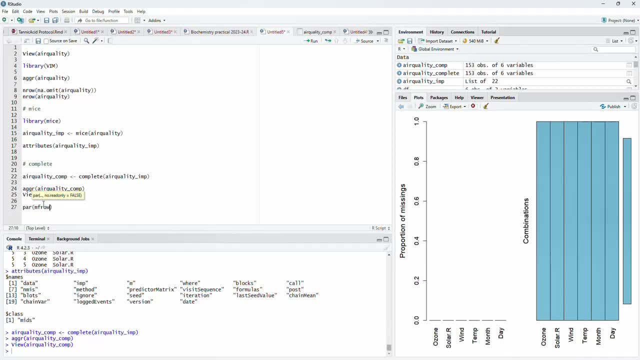 get me multiple graphs on same page. a metro is equal to C 2 by 2. will get 4 plots here and the first plot I will plot is box plot of air quality, original data, air quality, scalar ozone and of the name of the plot will be data with n a. 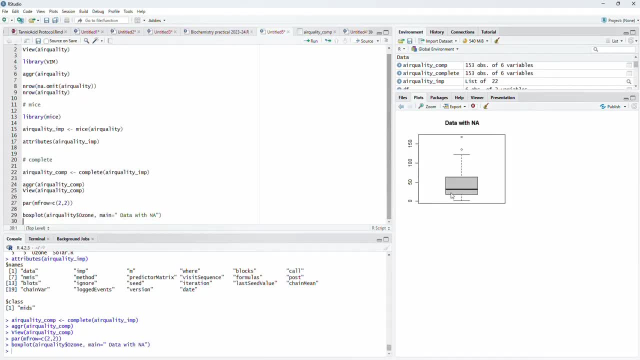 and run that. you can see here the box plot: distribution of the ozone data. and now we are going to use the distribution of the data and now we are going to use the distribution of the air quality scalar ozone. the Allāh aló so quality dot complete contains the imputed data set where no missing values. 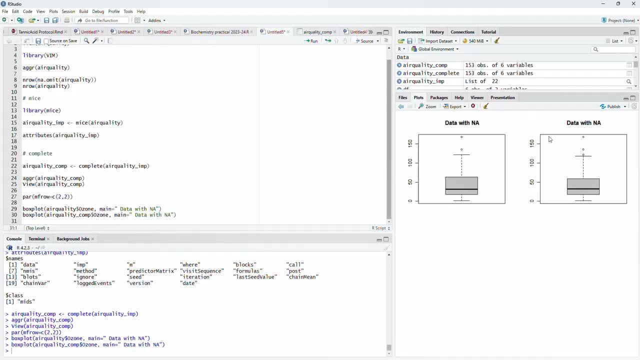 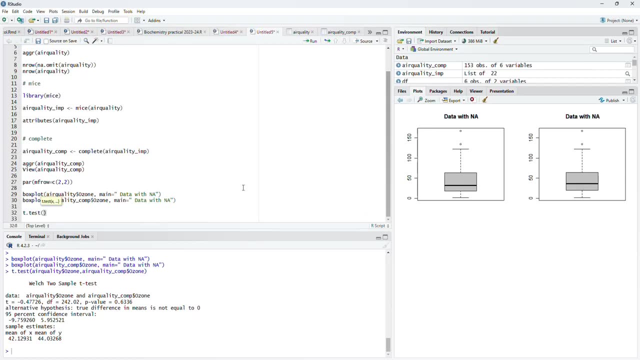 are there now and you can see that both are similar. we can compare quality of imputation using key test and will compare the data with missing values with the� data, with where we imputed those missing values, and we cannot run paired t test because some values are missing in this ozone and those are there in the completed data. therefore, pairing. 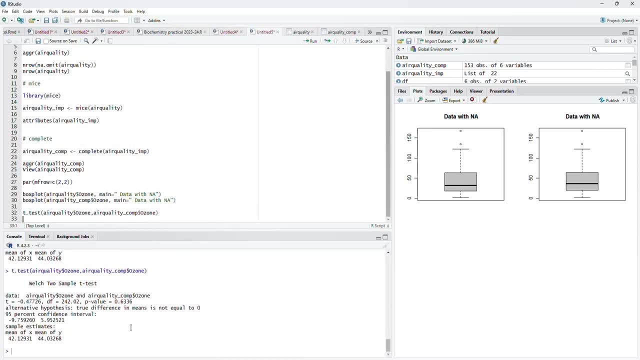 is not possible. when we run this test, you can see here we have got p value 0.6. our null hypothesis was: these two are not different. there is no difference between imputed and not imputed data. but here we are seeing the p value 0.6. that is above our critical value 0.05 and therefore we 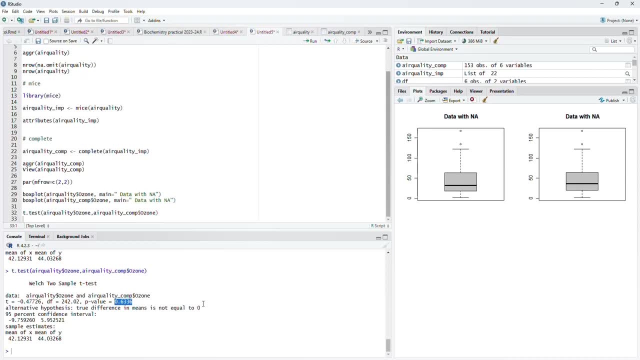 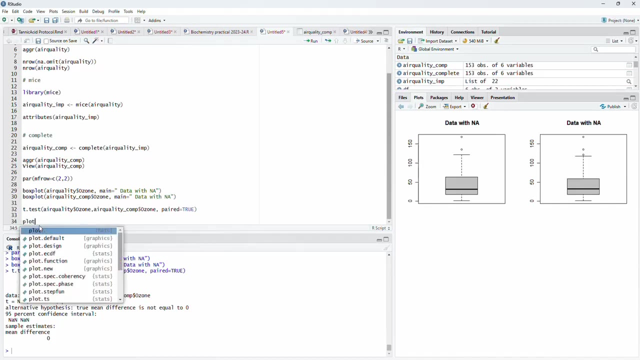 have to accept here that these two data sets are not different from each other and there is no effect of imputation, no worse effect of imputation on the actual data set we will visualize using the density plot also i will plot the density plot plot density of original data, air quality, ozone. and here we have to use that na dot rm also because 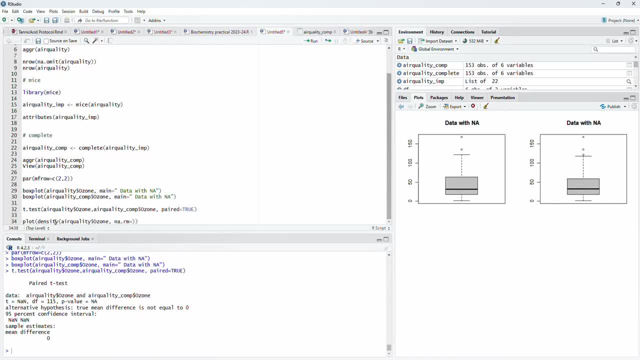 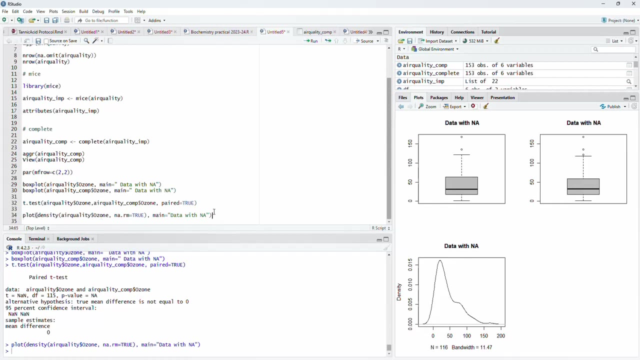 na values are there is equal to true and main will be data with na and we will run that now. this is there. now to this we will add the red line lines which will have the imputed or complete data. this main I will not carry here and just here. air quality, calm and the color. 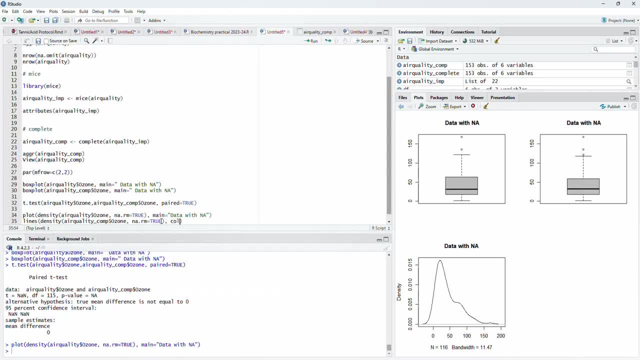 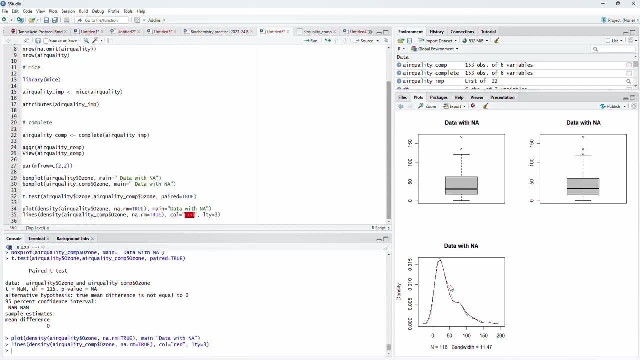 will change. that line should appear different and line type also will make dotted line and you can see that the original data with missing values and the complete data where missing values are imputed or both overlap quite nicely. and we can see the same for the solar are also just here I have to replace that with solar R and here also that will replace.